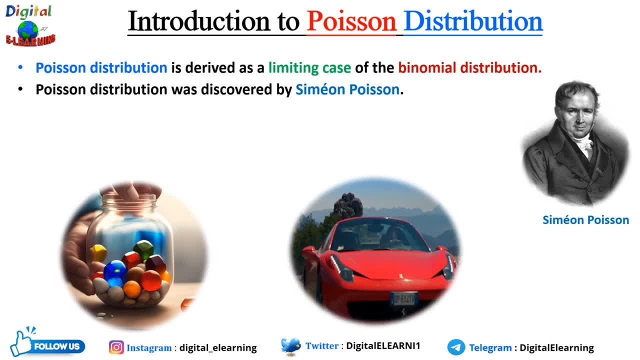 distribution can help us predict the probabilities of different number of cars passing by, based on the average rate of car arrivals. the poison distribution and the normal distribution are two most commonly used probability distribution in the statistics. I think you would have heard that these two are the most common probability distributions. 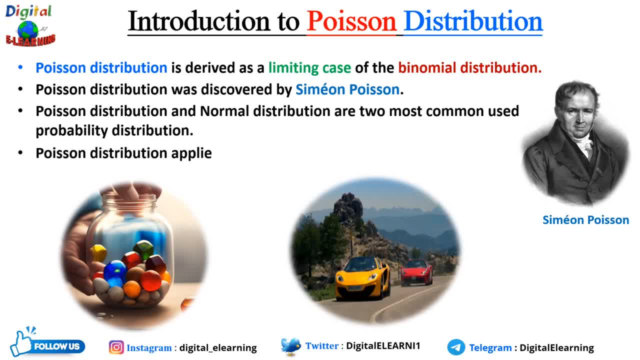 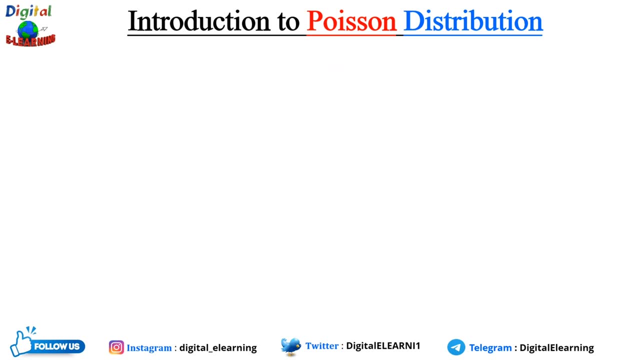 poison distribution applies to accident rates, arrival times, the defect rate, the occurrence of bacteria or fungus in the air and many other areas in the day-to-day life. now, when we talk about the shape of the poison distribution, it depends upon the parameter lambda, which represents the average rate of event occurring in a 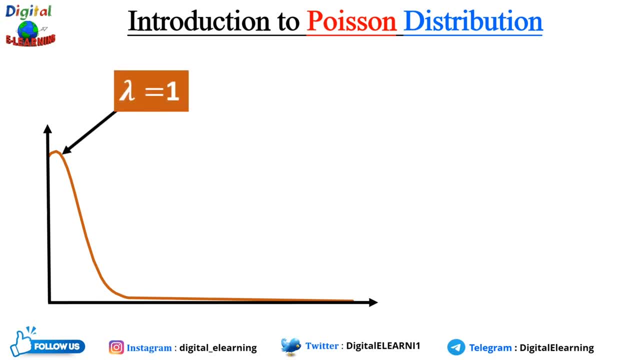 fixed interval. when lambda is small, say, for example, lambda equal to 1, the distribution is skewed to the right, with long tail on the right side. as lambda increases from 5 to 10, the distribution becomes more symmetrical and bell-shaped, resembling the shape of a normal distribution. 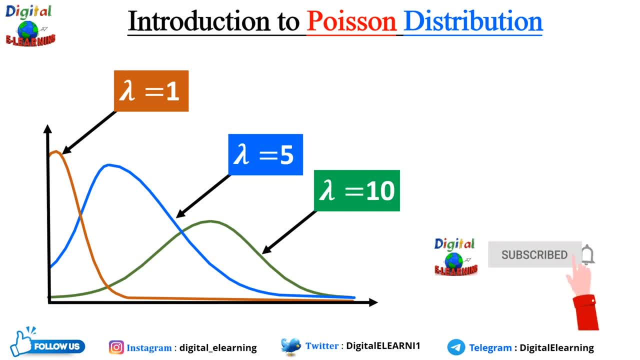 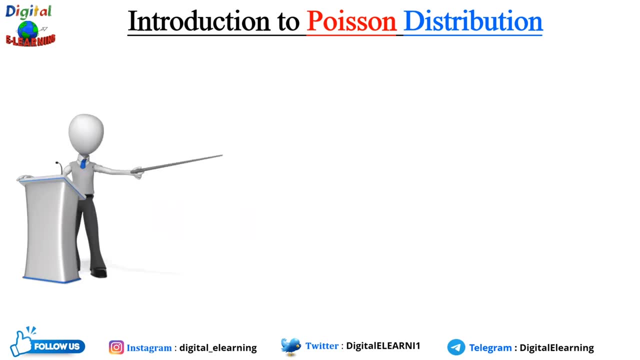 condition for poison distribution. so the poison distribution is derived as a limiting case of binomial distribution. under certain conditions: that the number of trials in the binomial distribution N is large and the probability of success in each trial p is small, The resulting distribution approaches the poison distribution To apply poison. 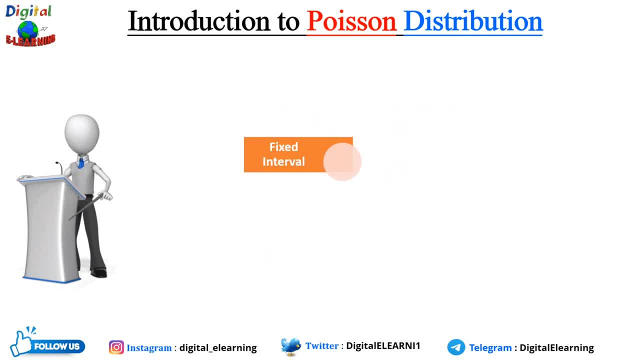 distribution. certain conditions should be met, like the fixed interval: The event of interest must occur within fixed interval of time, space and other discrete unit, For example counting the number of phone calls received in an hour and the number of accidents at particular insertion. 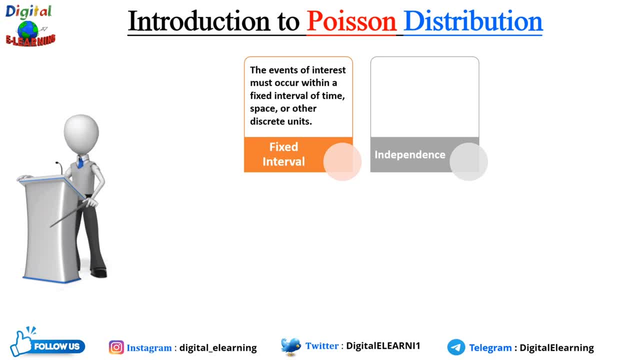 in a month. Independence: The occurrence of event must be independent of each other. This means that the happening of one event should not influence the likelihood of another event occurring. For example, the arrival of phone calls at call center should be random and not influenced by the previous. 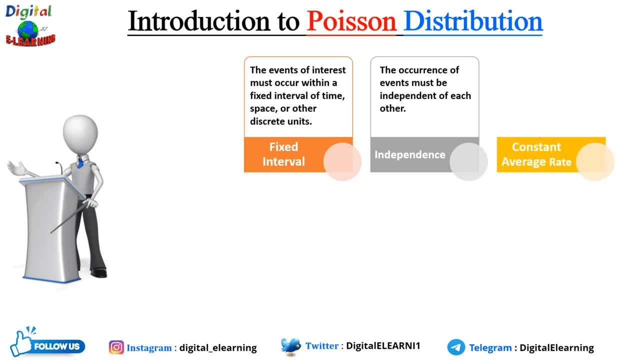 call Constant average rate. The average rate at which the event must occur remains constant over the entire period. The probability of an event happening in a given sub interval should be proportional to the length of that sub interval. For example, If an average rate is 3 accident per day, it should remain. 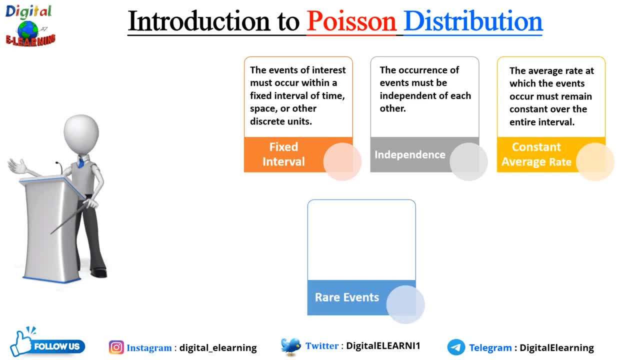 constant throughout the day. Rare events- The events of interest- should be relatively rare and have a low probability of occurrence. This condition ensures that the probability of occurrence remains constant throughout the day. ensures that the poison distribution is a suitable approximation, as it assumes that 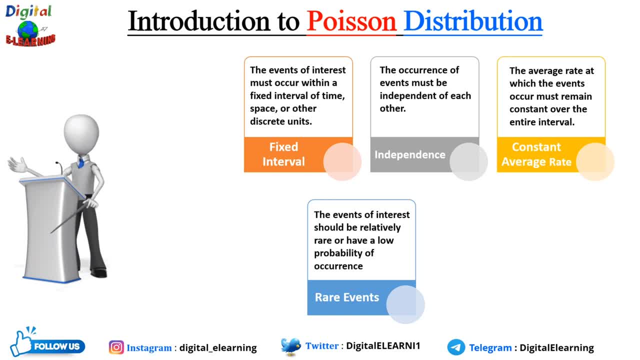 the probability of more than one event occurring in very small sub-interval is negligible. And last is the event count. The variable of interest is the count or the number of events that occur within the fixed interval. The poison distribution provides the probability of obtaining a specific count of events. It is important to note that the poison distribution 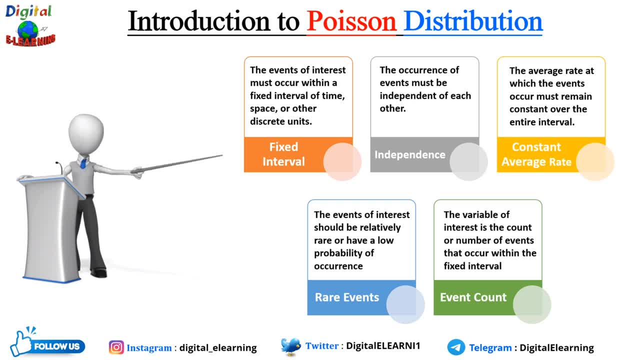 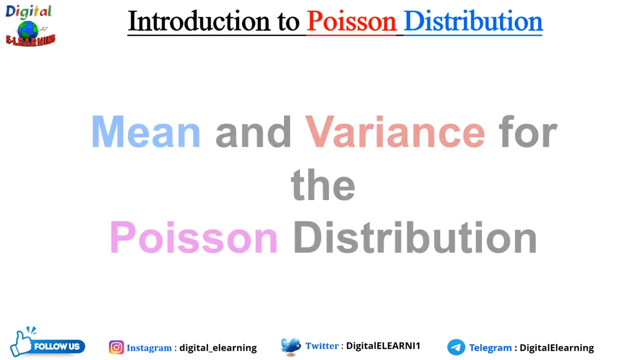 is an approximation and may not perfectly fit all situations. However, it often provides a good approximation for events that satisfy above conditions. Now let us see: how do we calculate mean and variance for the poison distribution? For that, let's first look at the poison distribution formula, where X denotes the count per second. 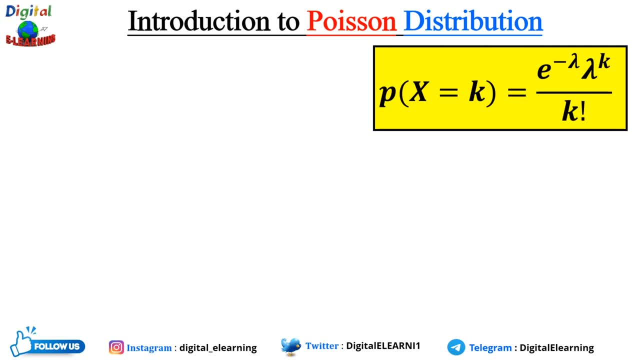 the probability that x is equal to k is given by e k power of minus lambda into lambda k power, k by k factorial, where lambda is the mean number of success, k denotes the number of success and e is a constant which is 2.718. when we come back to what is mean, mean is given mathematically. 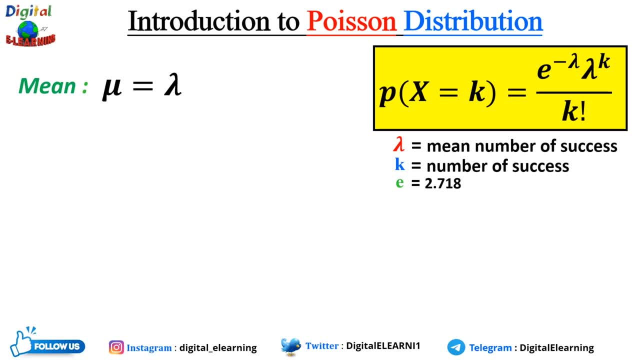 mu is equal to lambda. so mean represent the average or the expected number of events that occur within the fixed interval. now, what is variance? so variance of a population distribution is also given by lambda. so the variance represents the measure of spread or dispersion of distribution around the mean standard deviation: standard deviation is nothing but the under root of 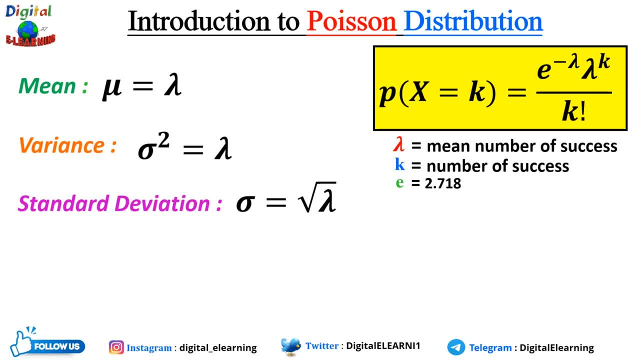 variance or lambda. so for poison distribution, mean and variance are equal and are both determined by parameter, lambda. so this means that if you know the average rate of events occurring, you can determine the expected mean and the variance of the distribution. now we can see this using some examples. let's look at some. 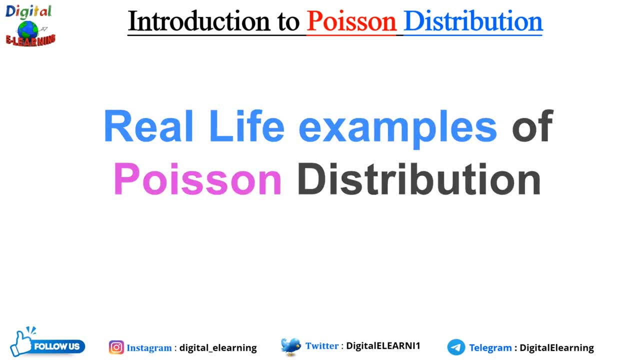 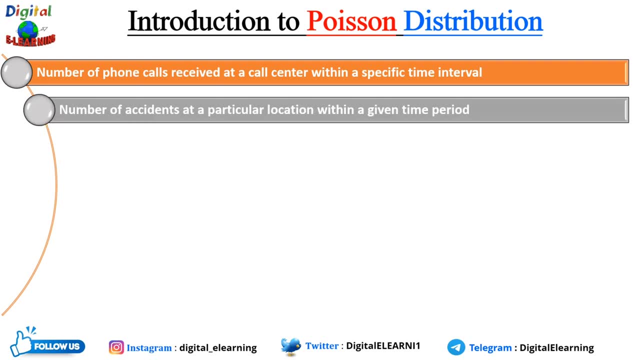 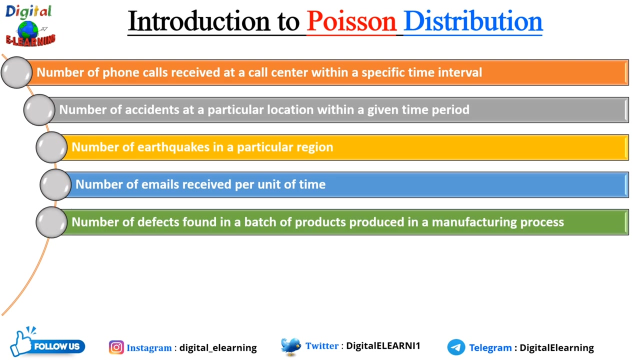 real life examples of the poison distribution: the number of phone calls received at the call center at time interval. the number of accidents at a particular location within a given time period. the number of earthquakes in the particular region. number of emails received per unit of time. number of defects found in a batch of product produced in a manufacturing process. 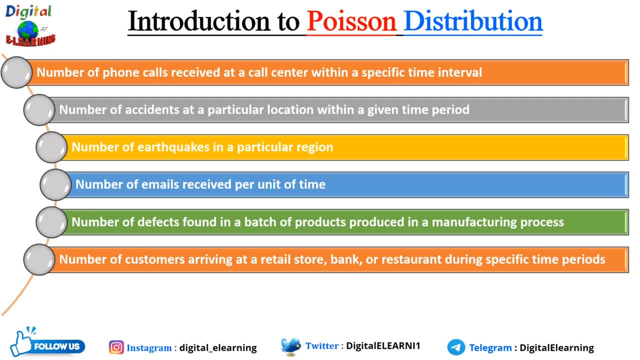 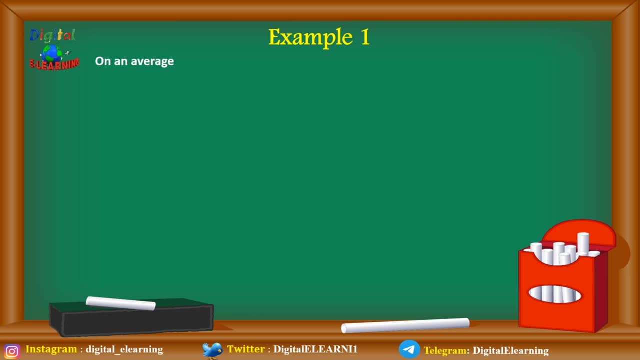 the number of customers arriving at retail store, bank or restaurant. the number of patients admitted to hospital or emergency room within a certain time period. these are some of the real life examples. so let's take the first example. on average, lightning kills three people every year in us. now we need to calculate what is the probability that 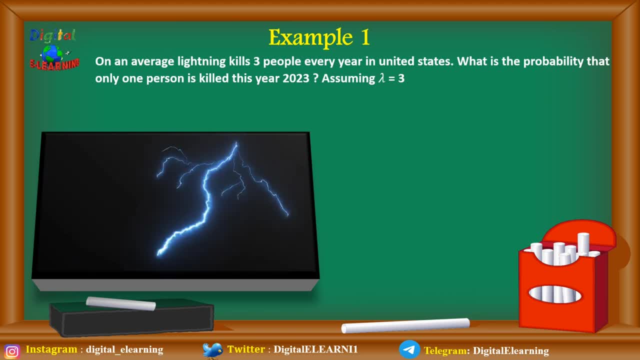 only one person is killed this year, assuming the lambda equal to three. so here we are, given that three people are killed on average in us, but we need to calculate that only one person is killed this year, not more than one. so we need to calculate that only one person is killed this year, not more than one. 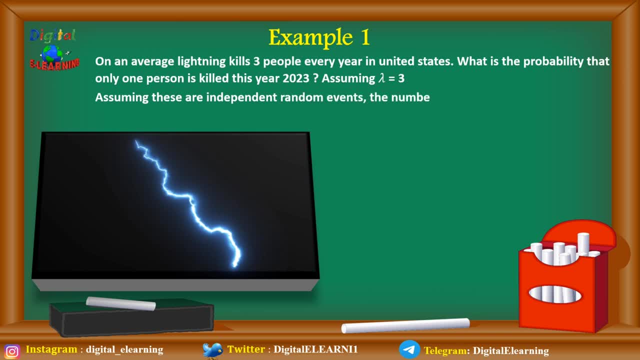 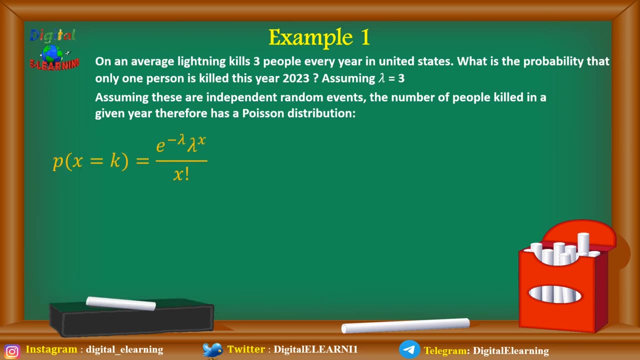 so in this case, assuming that they are independent, random events, as in what, how many people are killed last year, how many people will be killed this year- are totally independent, and that is why it follows the poison distribution. so we will use the formula: p is x equal to k, e power minus lambda. 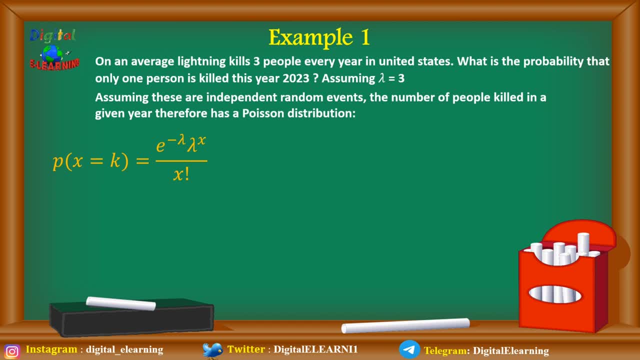 into lambda power x by x factorial. so we are assuming lambda equal to 3 here, which is given in the question, so we will put the values where lambda is equal to three. so we will put the values here where lambda is equal to expected. number of people killed: x is a number of people killed in. 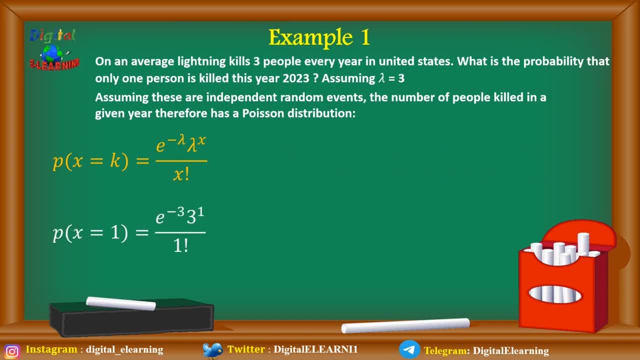 a year and we put the values for x equal to one, that is, one person is killed for e k power minus three into three k power, one by one factorial. we calculate, we get 0.15. so the probability is 15 percent that only one person will be killed this year. now let's take a little complicated example. 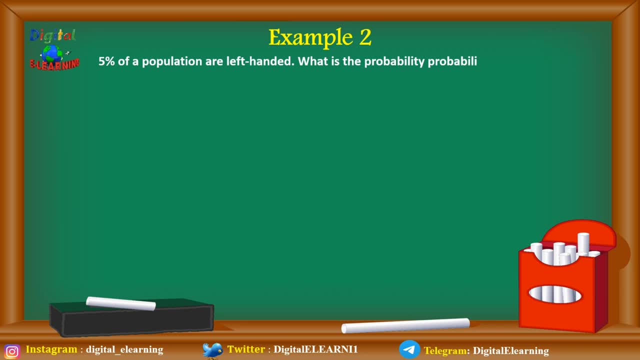 five percent of the population are left-handed. what is the probability that only one person will be killed this year? our probability that a random sample of 100 people contain, first case: zero left-handed people. second case: at most two left-handed people. third case: more than three left-handed people. we start with. 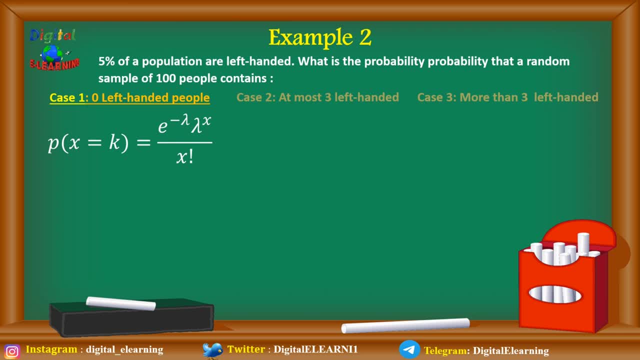 first case. here we have formula for poison distribution where x is a random variable that represents the number of left-handed people in a sample. k is the number of left-handed people who we are interested in. lambda is the mean of poison distribution, which is equal to n into p. 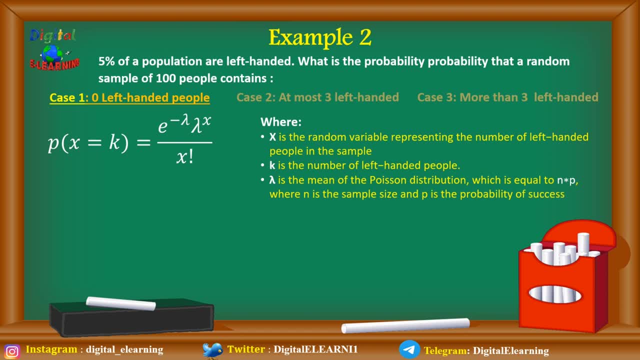 where n is the sample size and p is the probability of success, that is the proportion of left-handed people. now, in our case, k equal to 0. so lambda is equal to n into p, so that n is number of people, that is 100. probability of success is 5 percent, that is 0.05. so we get lambda is n into p as 5.. 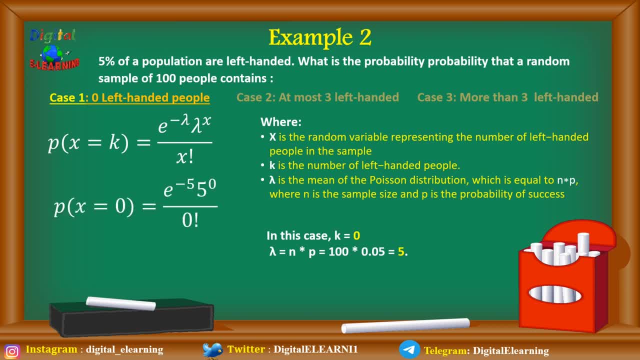 we put this value in the table or formula for poison distribution. for x equal to 0, we get ek power minus 5 into 5 k power, x divided by 0 factorial. so x is nothing but 0. here we put the values, we get 0.0067. 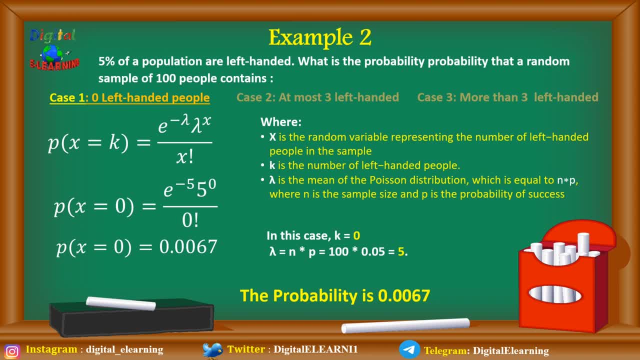 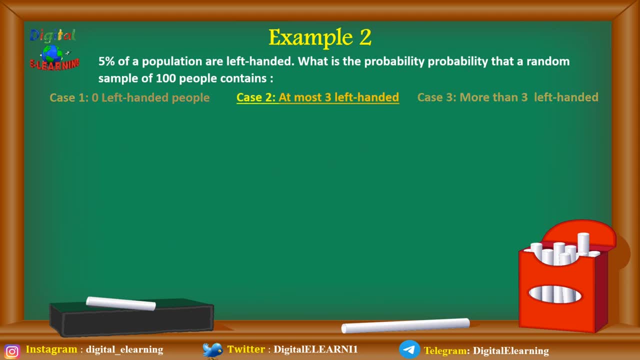 so the probability that comes out is 0.0067. we convert into percentage, we get 0.067 percentage. let's take the second case: at most three left-handed people. here we apply the same formula for poison distribution: we get 0.067 and we get 0.067. we convert into percentage, we get 0.067. 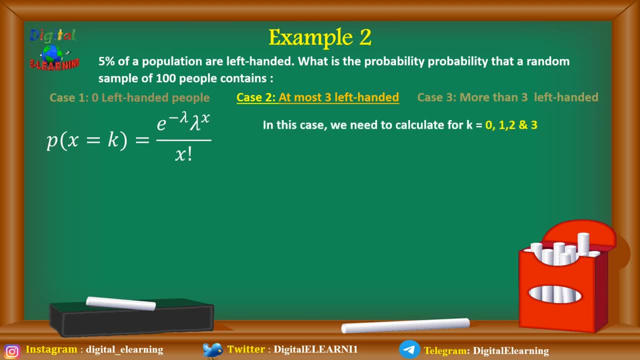 of our person distribution. in this case, we need to calculate for k equal to 1, 2 and 3, because we the case talks about at most three left-handed persons. so this includes zero definite people, one definite people, two and three as well- lambda, as usual- will have same value: five. so this is what. 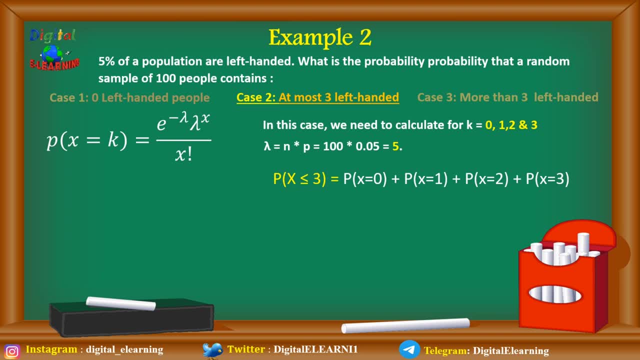 we need to calculate. we will calculate for x equal to zero, one, two and three, and add all at the ml we already done for x equal to zero in the previous example. we start with x equal to 1, which get 0.0337. for x equal to 2, we get 0.0842. for x equal to 3, we get 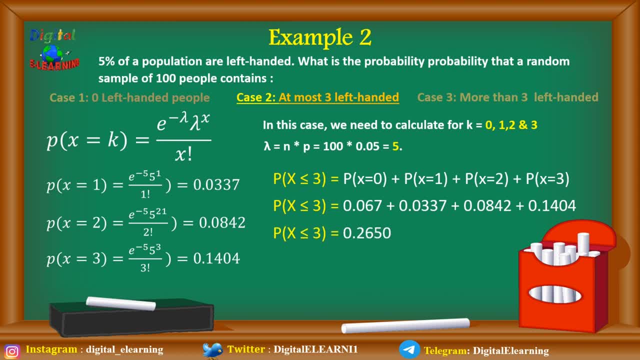 0.1404. we put this here and we sum it up, we get 0.2650. the probability that the population contains at least at most three left-handed is 0.2650. if you convert into percentage, it comes to 26.5. let's take the third example. let's take the third example. 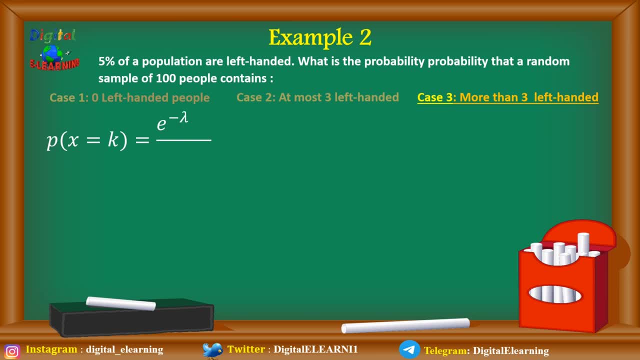 we have more than three left-handed people again apply the same formula for poison distribution, but in this case we need to calculate for k greater than equal to 3, not equal to, but k greater than 3. so we have the same lambda as np. we get 5.. so this is what we need to calculate for x greater. 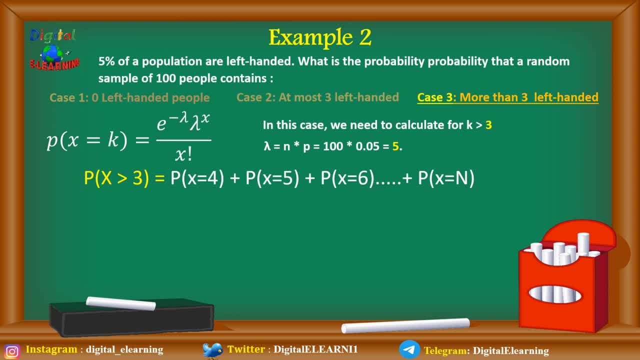 than equal to 3.. so we need to calculate for 4, 5, 6 and so on till n, which is difficult to calculate. the other way is we know that the sum of probability is always equal to one. So we, for x equal to 3, will subtract it from 1, which is less than equal to 3.. 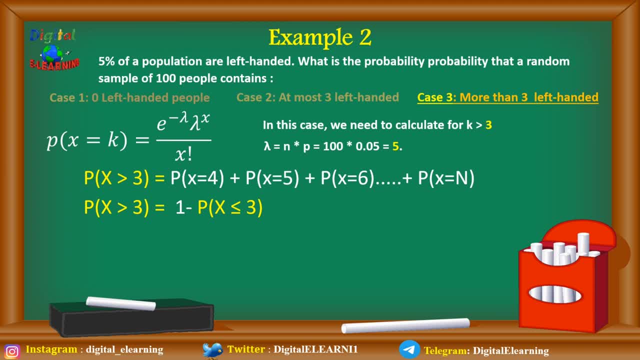 So that p x less than equal to 3 that we have calculated in the previous case 2, you can look at that and if we subtract from 1, we get p- all the values, which is more than 3.. So we subtract, we get as p greater than 3 equal to 0.7350.. 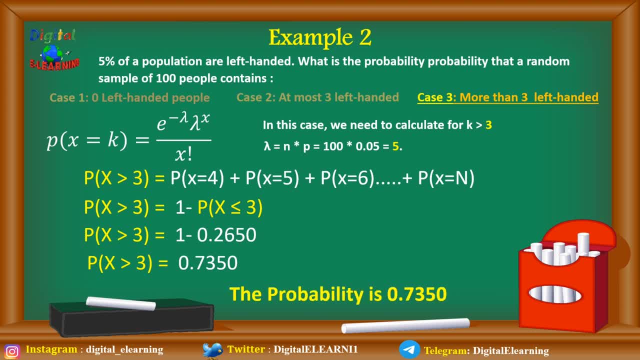 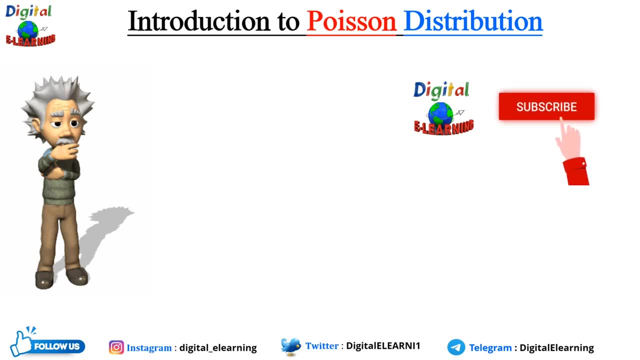 So probability that comes up is 73.5.. So if you are still watching this video, don't forget to hit the subscribe button and do press the bell icon for all the notification from Digital E-Learning. And if you like this video, don't forget to hit the like button as well. 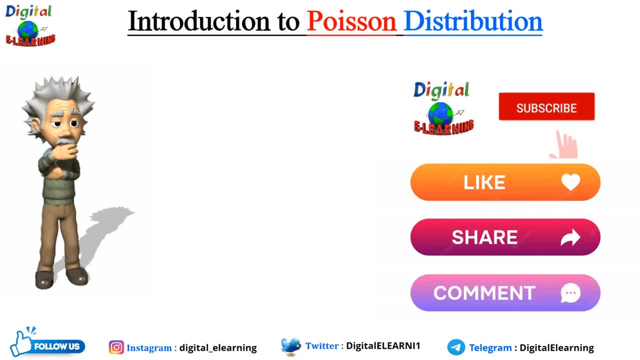 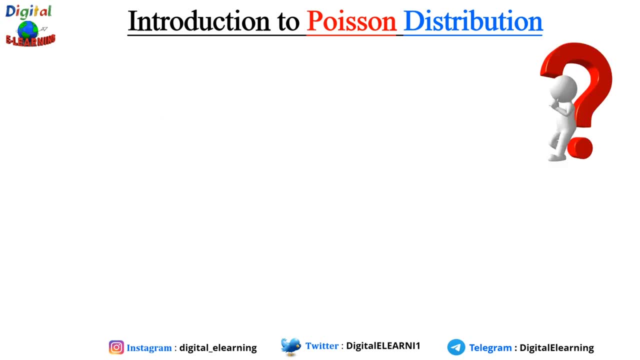 Share this video with all your friends and colleagues And in case if you have any suggestions or comment, do let me know in the comment box below. Now is the quiz time on this topic. First question: The mean of poison distribution is equal to.